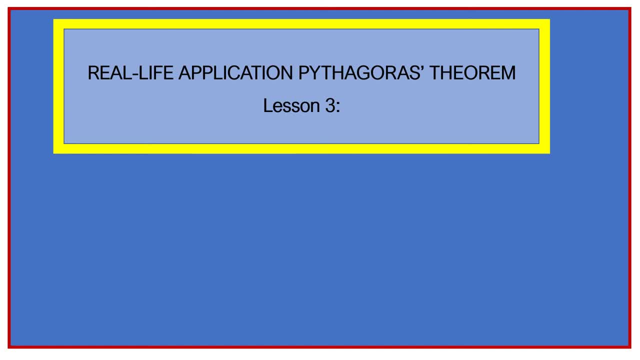 Welcome to lesson number three, And today we are going to learn about real-life application of Pythagoras' theorem. In case you did not watch lesson one and two, you can check in the description part and click on the links below. So for now, let's continue with our lesson. 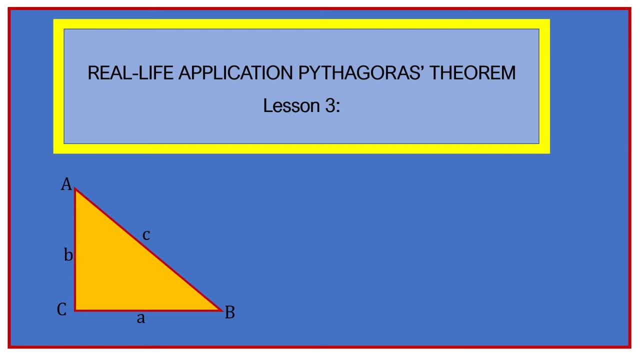 Remember, Pythagoras' theorem only applies to right-angled triangles, And for this case we have got a right triangle, ABC. So we need to know that the hypotenuse is AB, which is the longest side of the triangle. So in that case we say AB squared equals BC squared plus AC squared, And then this can be. 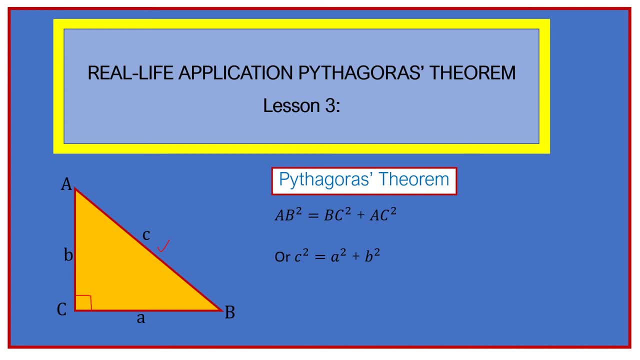 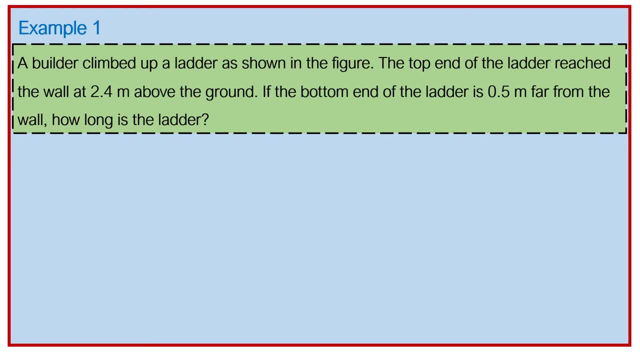 the same as C squared equals A squared plus B squared. Let us now look at example one. A builder climbed up a ladder. as shown in the figure, The top end of the ladder reached the wall at 2.4 meters above the ground. 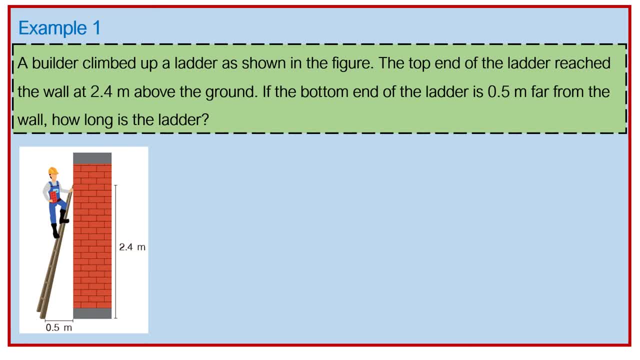 If the bottom end of the ladder is 0.5 meters far from the wall, how long is the ladder? So we need to know how long is this ladder. We see that The distance between the wall and the ladder is 0.5 meters. 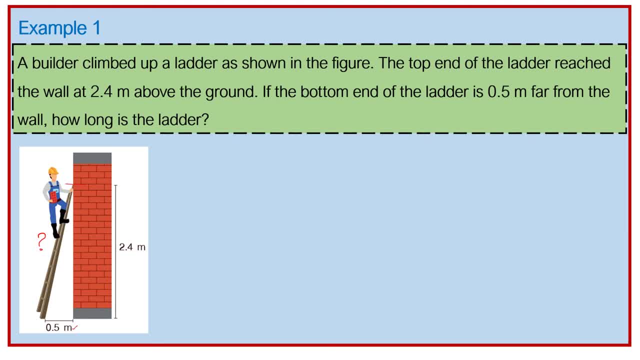 And the ladder moved and covered 2.4 meters from the ground. So you can see that this scenario forms a right triangle And for that case we need to know the hypotenuse. So since this is a right triangle, we can use the Pythagoras' theorem. 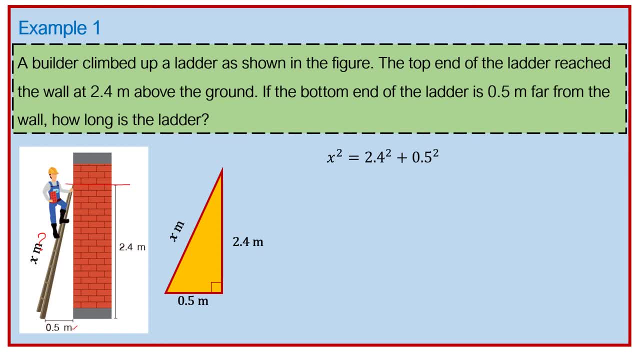 So we get X squared equals 2.4 squared plus 0.5 squared To get 5.76 plus 0.25 and we get 6.01.. Then, since we need to know the hypotenuse, know the length of the ladder, It can't be a negative, so that's why we will take the positive. 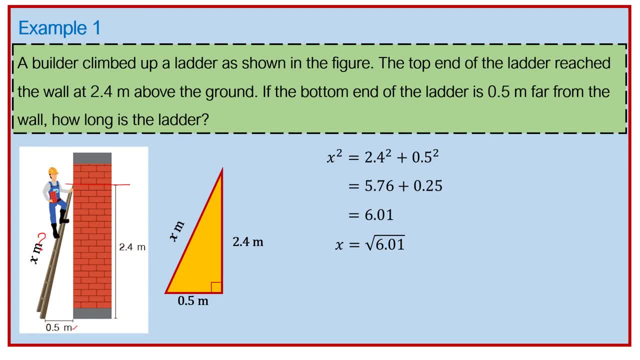 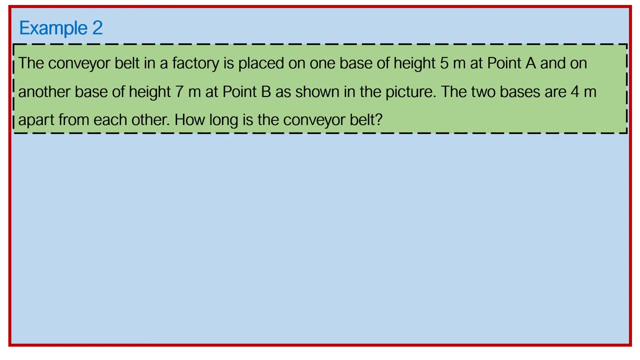 square root of 6.01, and for that case we get the approximate length of 2.45.. Therefore, the ladder is approximately 2.45 meters. Let us move on with example 2.. The conveyor belt in a factory is placed on one base. 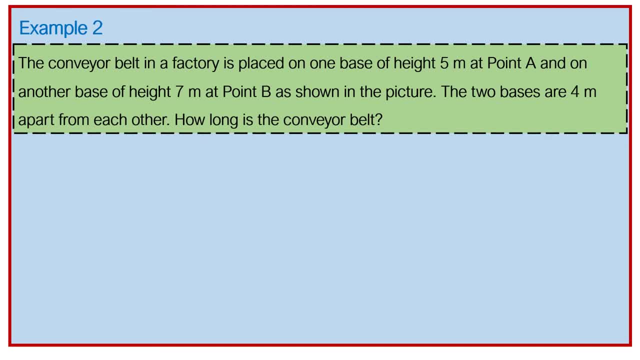 of height 5 meters at point A and on another base of height 7 meters at point B, as shown in this picture. You can see we have two bases. one base is A and another base is B. B is 7 meters from the ground and A is 5 meters from the ground. okay, so base A and B. 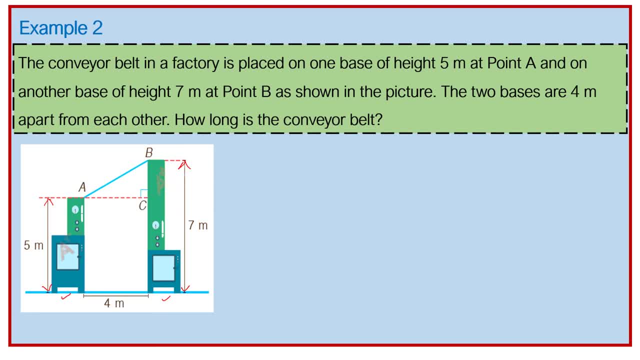 they are 4 meters apart, 4 meters. so you can see that we are forming a right triangle. we are forming a right triangle whereby this is a, this is C and this is B, so you can see that AC is 4 meters and BC it is 7 minus 5, which is equal to 2.